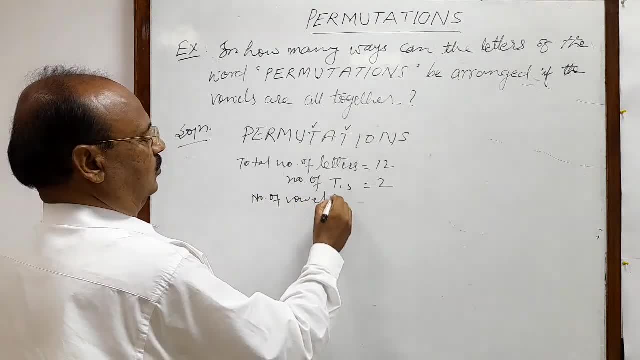 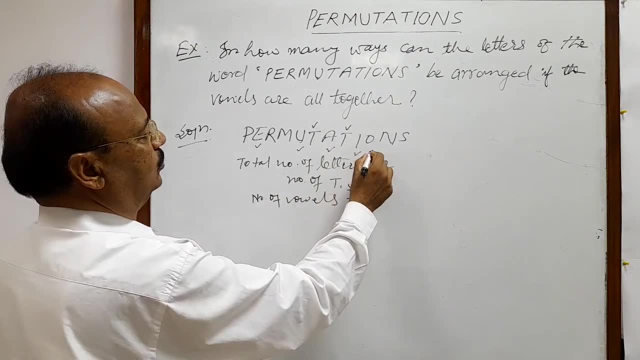 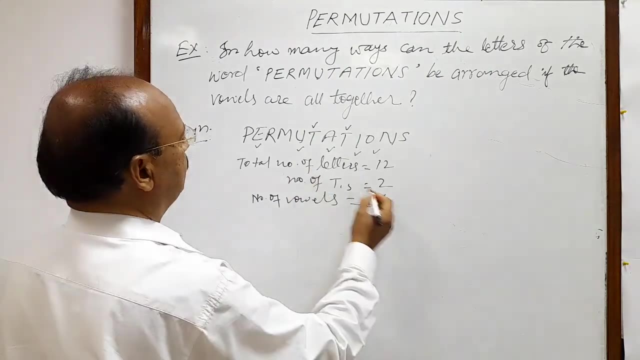 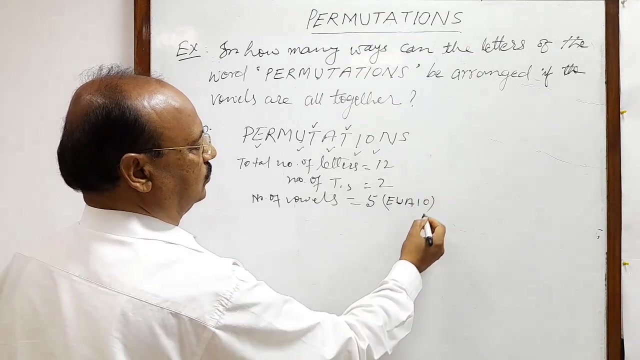 Number of vowels is how many Number of vowels? This is 1,, 2,, 3,, 4, 5.. There are 5 vowels, Which are 5 vowels are E, U, A, I and O. So, very interestingly, all the 5 vowels are here. 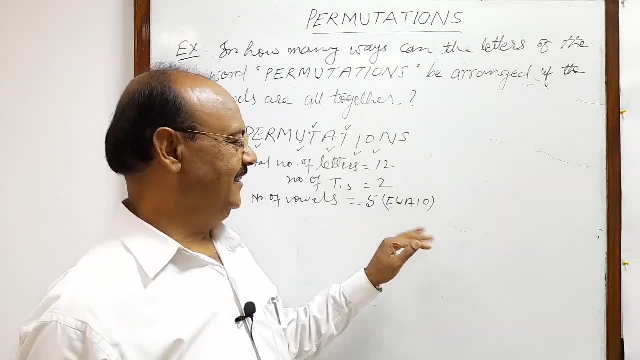 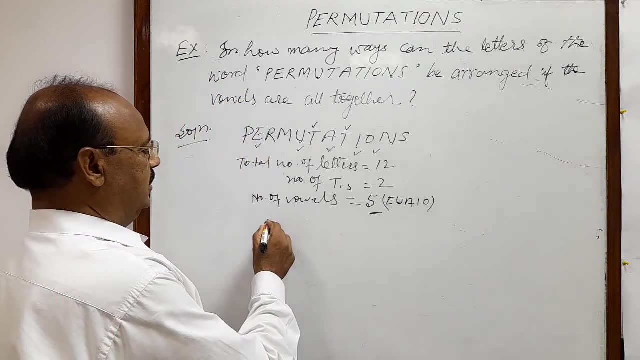 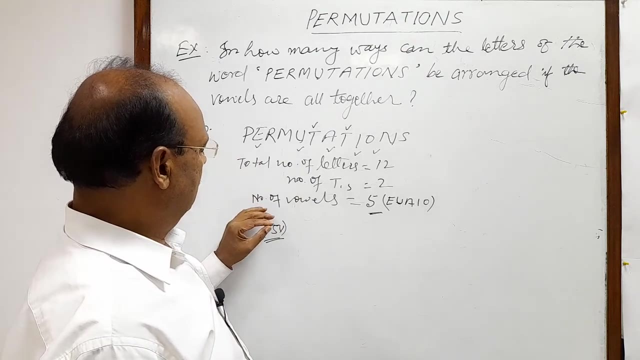 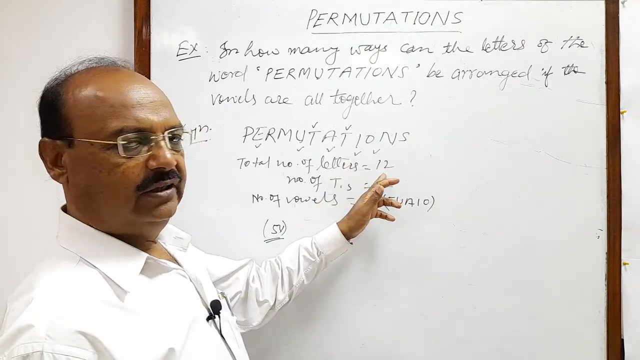 A, E, I, O, U. All the 5 vowels are here. Very interesting question. Okay, So this is the condition that these 5 vowels will always remain together. So, after keeping these 5 vowels together, how many other letters are there? Total letters are 7.. And 5 are vowels, So other letters are 7.. Okay, 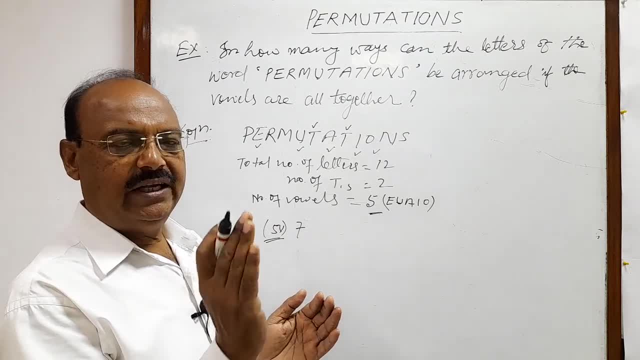 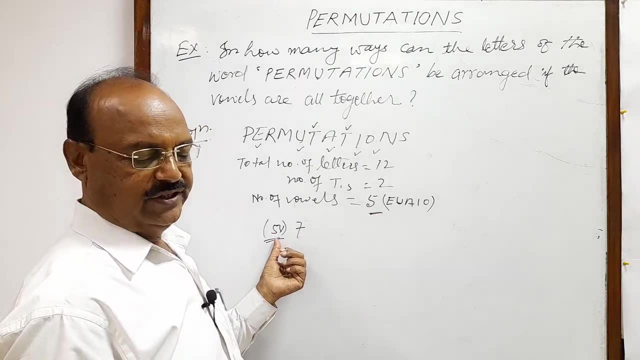 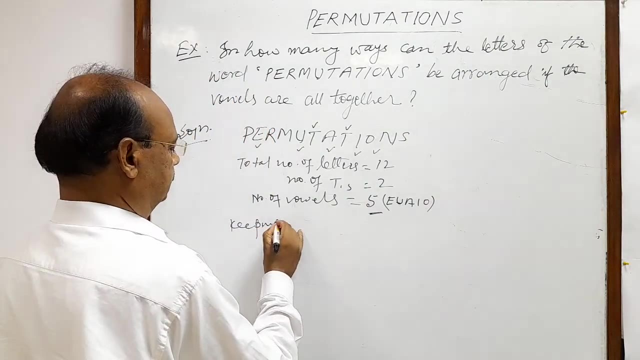 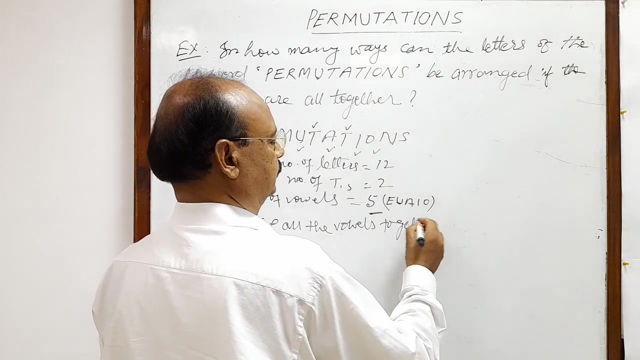 five vowels will be in one group, so it will be treated as a single object, and other seven letters are here, so total number of objects under this case will be seven plus one, eight, correct? so let us write here keeping all the vowels together, taking as one object. 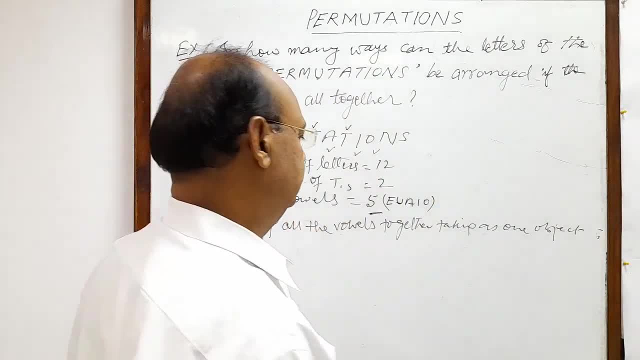 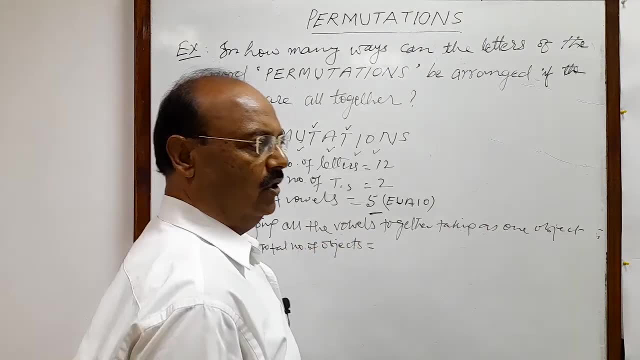 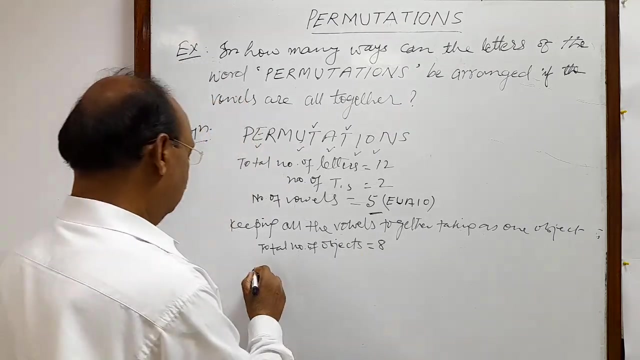 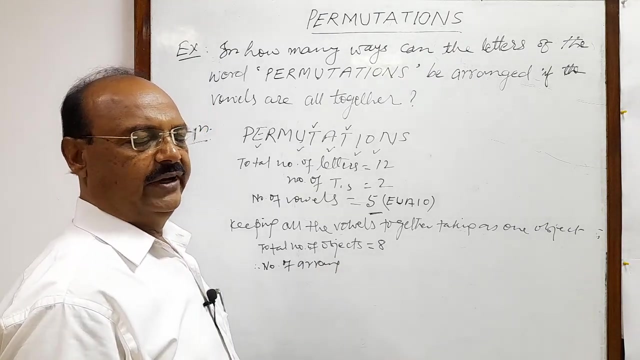 and rest of the objects are different. total number of objects: how many? all five vowels will be treated as one object and remaining seven letters, so seven plus one eight. so therefore, number of arrangements means number of words, form with or without meaning. when all the vowels will be kept together, number of arrangements total. 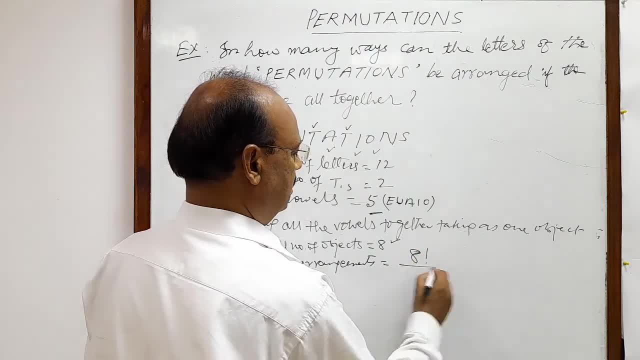 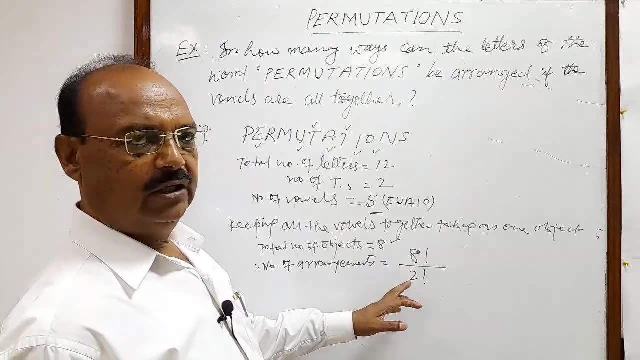 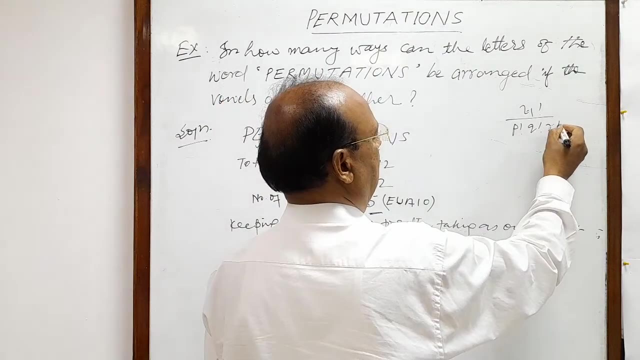 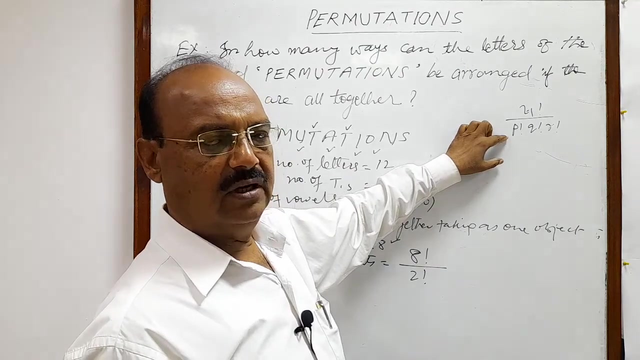 arrangements. object is 8, so 8 factorial divided by 2 factorial, isn't it How? 8 factorial by 2 factorial? Because we have discussed several times a formula n factorial by p factorial, q factorial, r factorial, when total number of objects is n and there are p alike objects of.